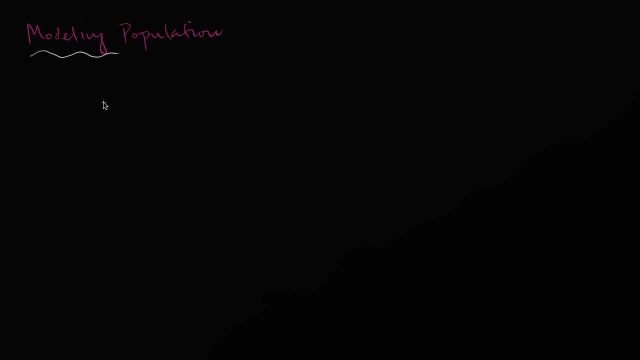 but we're going to get there using the power of modeling with differential equations. So let's just define some variables. Let's say that p is equal to our population, And let's say that t is equal to the time that has passed in days. 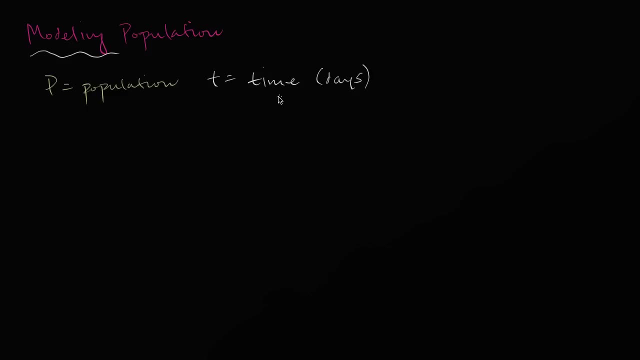 In days. It could have been years or months, But let's say we're doing the population of insects that reproduce quite quickly. So days seem like a nice time span to care about. Now, what would be a reasonable model? Well, we could say that the rate of change of our population with respect to time 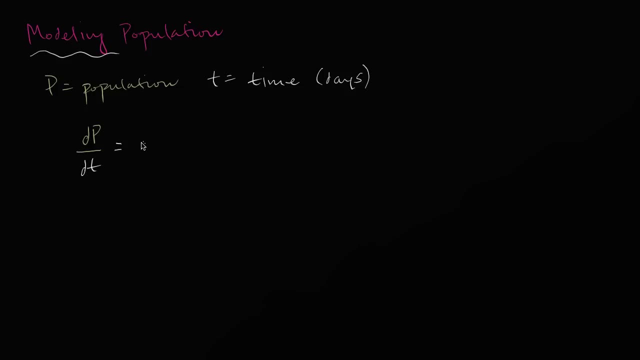 is well a reasonable thing to say is that it's going to be proportional to the actual population, The actual population. Why is that reasonable? Well, the larger the population, the larger the rate. at any given time, If you have a thousand people, the rate at which they're reproducing is going to be more. 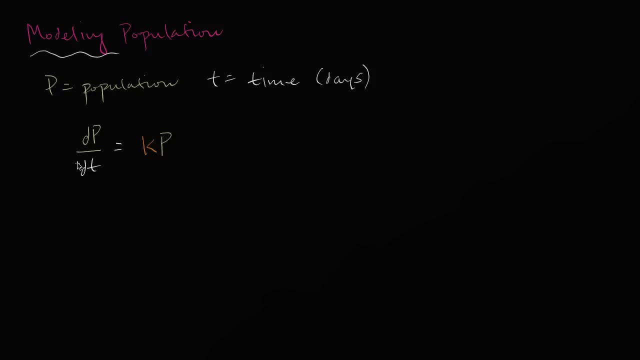 or a thousand insects is going to be more insects per second or per day or per year than if you only have ten insects. So it makes sense that the rate of growth of your population with respect to time is going to be proportional to your population. 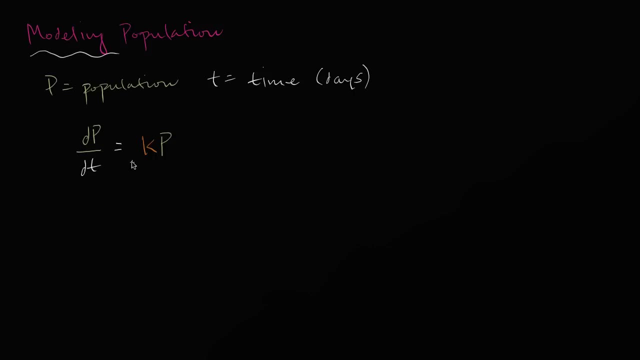 And so you know, sometimes you think of differential equations as these daunting, complex things. but notice, we've just been able to express a reasonably not so complicated idea. The rate of change of population is going to be proportional to the population. And now, once we've expressed that, we can actually try to solve this differential equation. 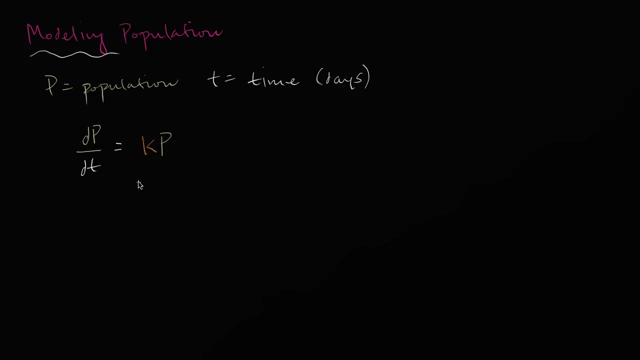 find a general solution and then we could try to put some initial conditions on there or some states of the population that we know to actually solve for the constants to find a particular solution. So how do we do that? And I encourage you to pause the video at any time- 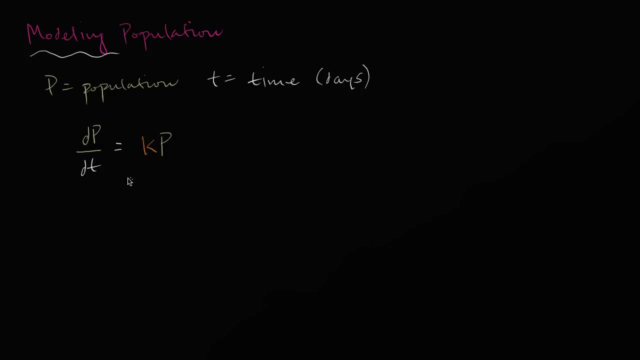 and see if you can solve this differential equation. So assuming you at least maybe have had an attempt at it And you might immediately recognize that this is a separable differential equation. And in separable differential equations we want one variable and all the differentials involving that variable on one side. 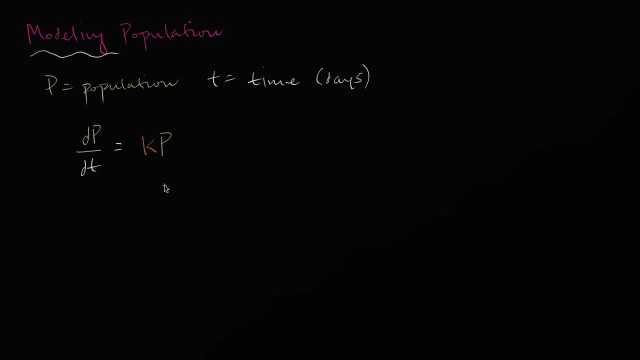 and the other variable and all the differentials involving the other variable on the other side, and then we can integrate both sides And, once again, the derivative of p with respect to t. this isn't quite a fraction. This is the limit as our change in p over change in time. 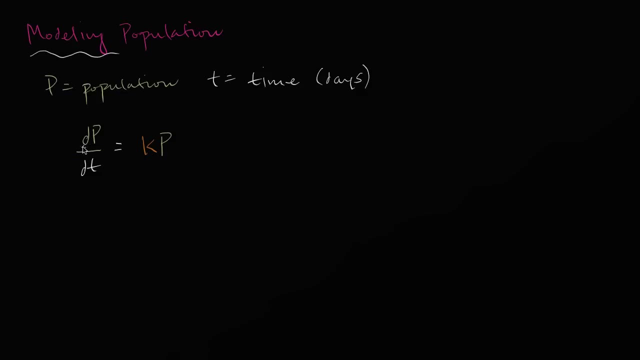 This is our instantaneous change, but for the sake of separable differential equations, or differential equations in general, you can treat this derivative in Leibniz notations like fractions and you can treat these differentials like quantities, because we will eventually integrate them. 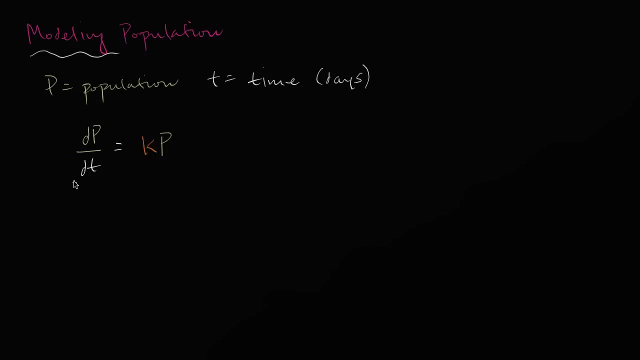 So let's do that. So we want to put all the p's and dp's on one side and all the things that involve t or that I guess don't involve p, on the other side, So we could divide both sides by p. 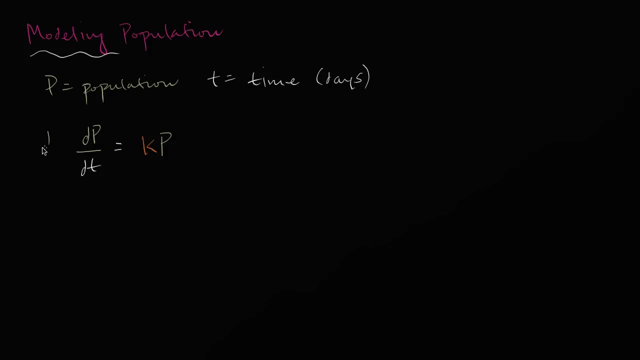 We could divide both sides by p, And so we'll have 1 over p. You have 1 over p here, and then those will cancel, And then you could multiply both sides times dt. We could multiply both sides times dt, Once again treating the differential like a quantity. 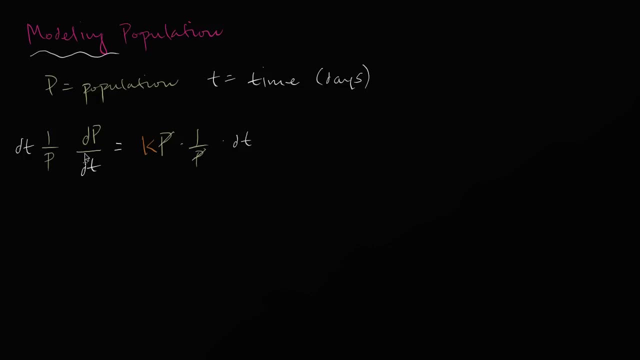 which really isn't a quantity. You really have to view this as a limit of change in p over change in time, The limit as we get smaller and smaller and smaller changes in time. But once again, for the sake of this, we can do this. 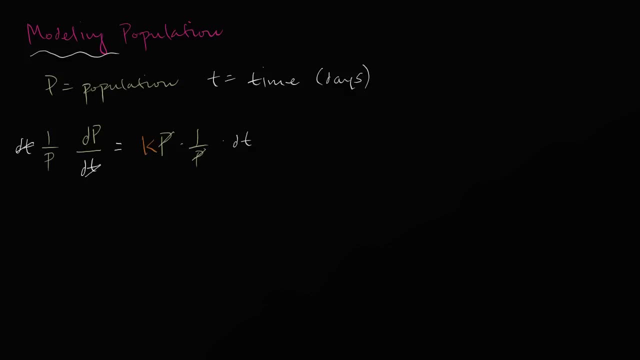 And when we do that, we would be left with 1 over p. dp is equal to k, dt Is equal to k dt. Now we can integrate both sides Because this was a separable differential equation. we were able to completely separate the p's and dp's. 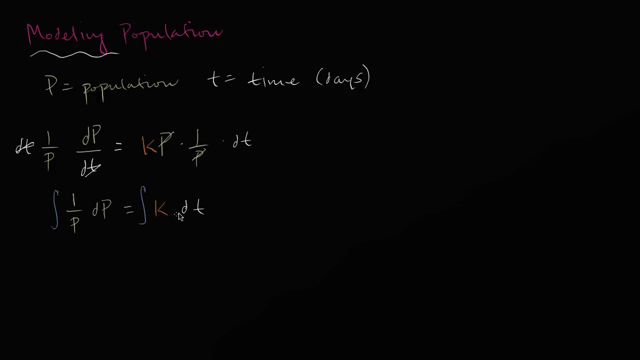 from the things involving t's or, I guess, the things that aren't involving p's, And then, if we integrate this side, we would get the natural log of the absolute value of our population And we could say plus some constant if we want. 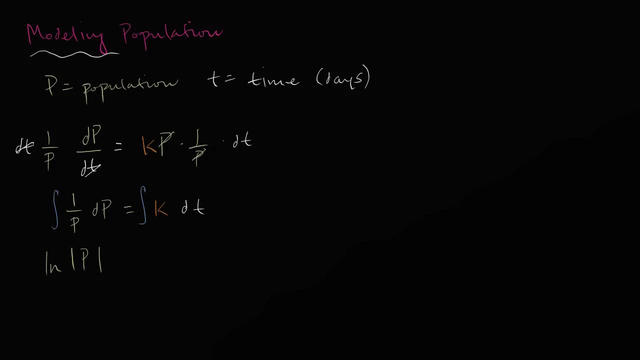 but we're going to get a constant on this side as well. So we could just say that's going to be equal to, that's going to be equal to k times t plus some constant. I'll just call that c1. And once again I could have put a plus c2 here. 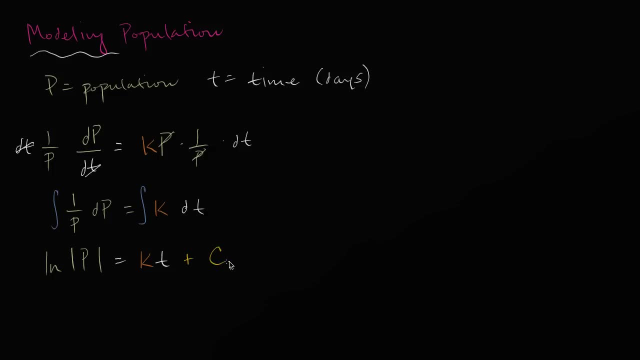 but I could have then subtract the constant from both sides and I would just get the constant on the right hand side. Now, how can I solve for p? Well, the natural log of the absolute value of p is equal to this thing right over here. 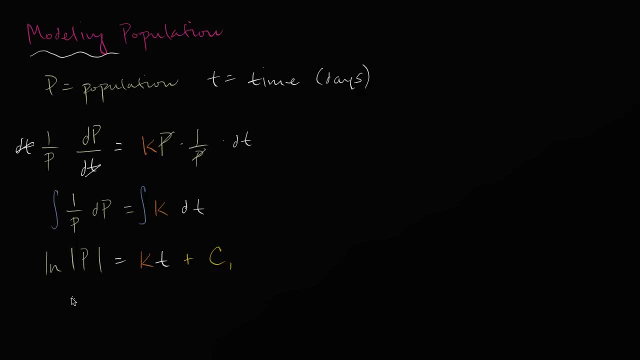 That means that's the same thing. that means that the absolute value of p, that means that the absolute value of p is equal to e, to all of this business, e to the, e to the. let me do the same colors: kt plus c1.. 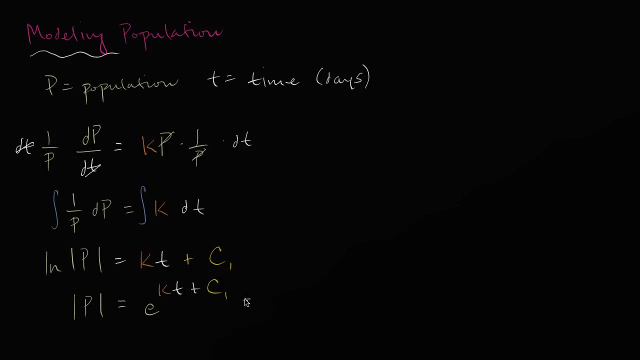 Now this right over here is the same thing, just using our exponent properties. this is the same thing as e to the kt, e to the k, times, t times e, times e to the c1, e to the c1.. Now this is just e to some constant. 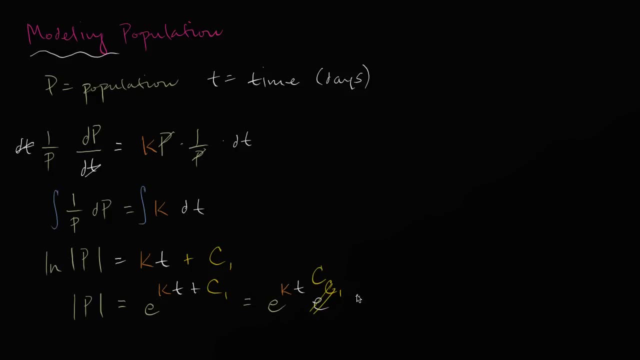 so we could just call this, let's just call that the constant c. So this is all simplified to ce, ce to the kt, to the kt, And if we assume our population at any given time is positive, then we could get rid of this absolute value sign. 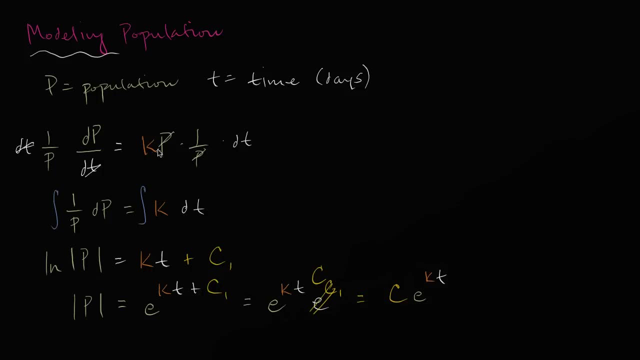 Now we have a general solution to this, frankly, fairly general differential equation. we just said proportional. we haven't given what the proportionality constant is, but we could say, if we assume positive population, that the population is going to be equal to some constant c times e. 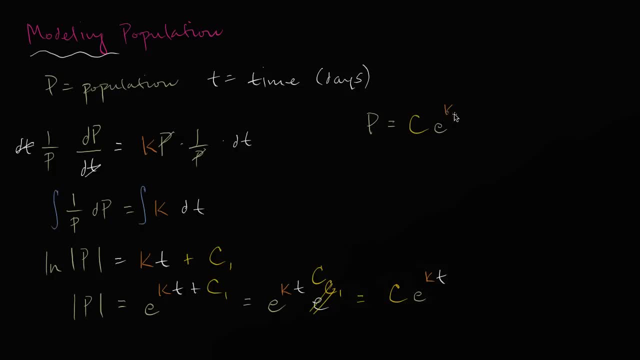 e to the kt power to the kt power. And the reason why I said that you've seen this before is this is just an exponential function and it's very likely that in algebra or in precalculus class you have modeled things with exponential functions.